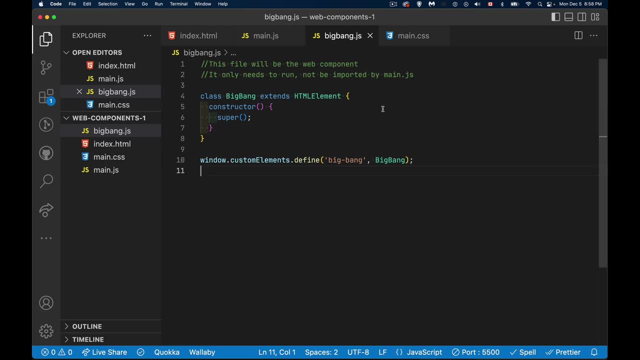 On the bigbang file. there's no exporting of this, So we just have to run the script And it's this bottom line right here that we've got Window, custom elements and window is the global object. We can even leave that off, We can just say: custom elements, dot define big bang, big bang. 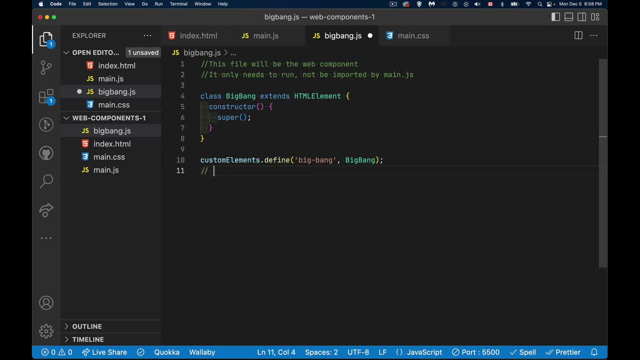 This first one, that is, the tag. So we are building something like this. I can now put a big bang element on my page. You can decide what you want these names to be. There has to be a hyphen in the name, though. 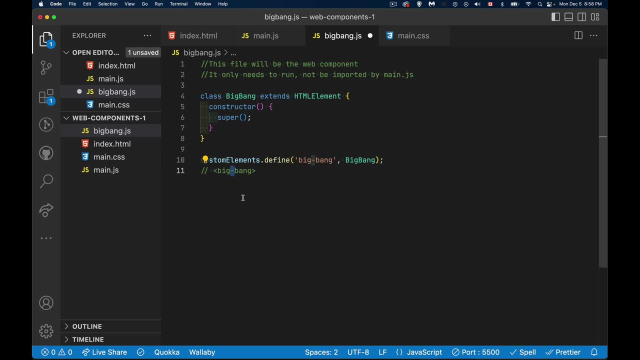 This is one of the things that makes it stand out as a custom element. Whatever the name is that you choose, there needs to be a hyphen in the name somewhere, So we're defining this as our tag, our custom element, And this right here, this class. this is the thing. 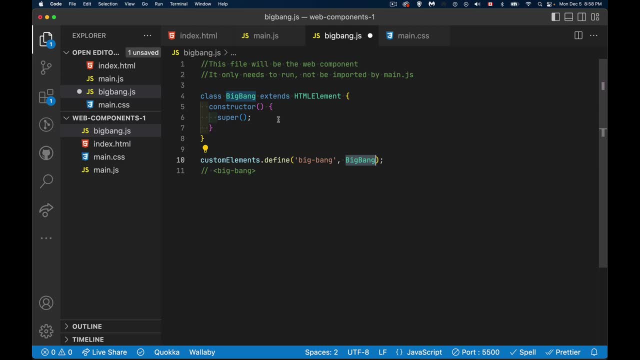 that's going to build our actual element. So inside of here we've got our constructor that runs And anytime somebody adds one of these things to the page, we're going to be creating one of these things. So this class gets run, the constructor gets run to define what one of these 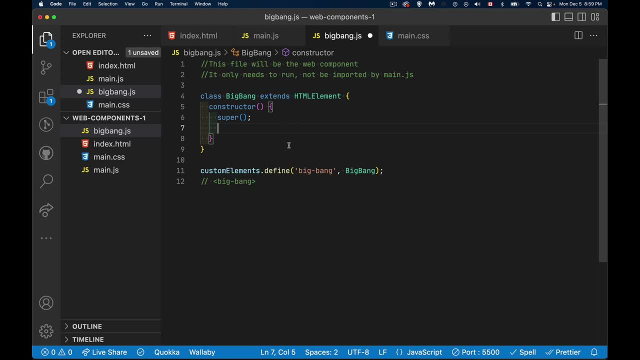 is, Every time you add one to the page, we're running the constructor. We're saying, hey, I need another one of those things Inside of here. one of the things that we need is is a shadow root, So this is like the container that's going to hold. 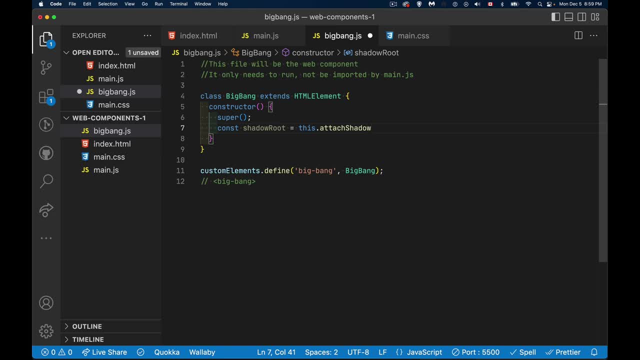 your component- Custom web components- because they can contain styling, because they can contain scripts and functionality and behaviors. we don't want those things spilling out and impacting the rest of the page. I don't want to define CSS in here and have it change the way the rest of the page looks. The other way is fine. 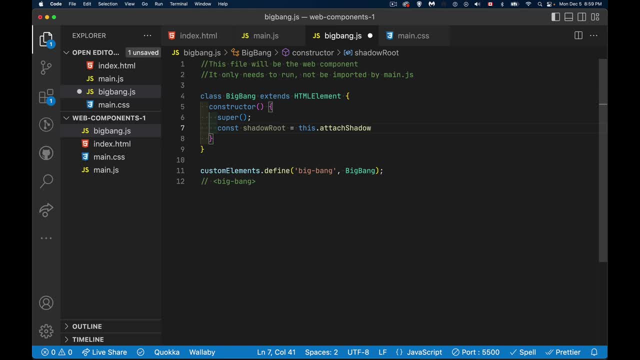 The rest looks beautiful. The other way just cells them all out and completely ruins everything of the page. can have its styles cascade down into our page, into our component, but we don't want to affect the rest of the page. so the shadow root, we're attaching a shadow, so wherever we're putting 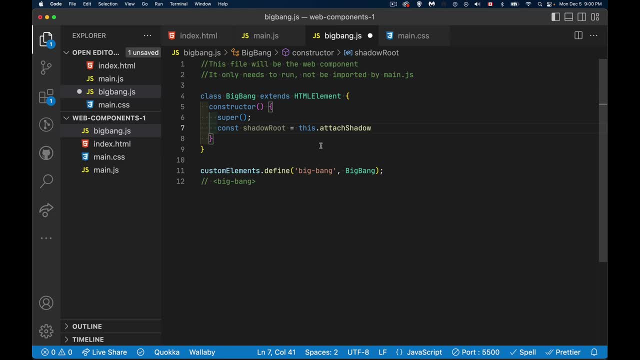 this thing on the page. there's this container, this shadow root that is put on there and it sort of creates a sandbox around our element when we call attach shadow. there's one thing that we have to pass in here, one setting, so it's an options object and the setting is mode and it can be open or it. 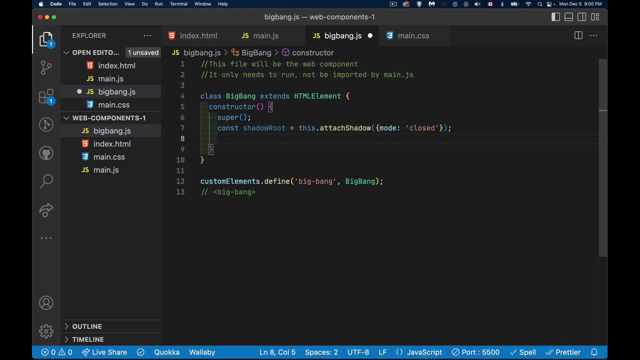 can be closed. open means that the parent script mainjs can actually do things like document dot query selector and get inside of our element and see what the actual tags are that we're using inside of our custom component. if it's closed, they can't. that's it. that's all we're saying. 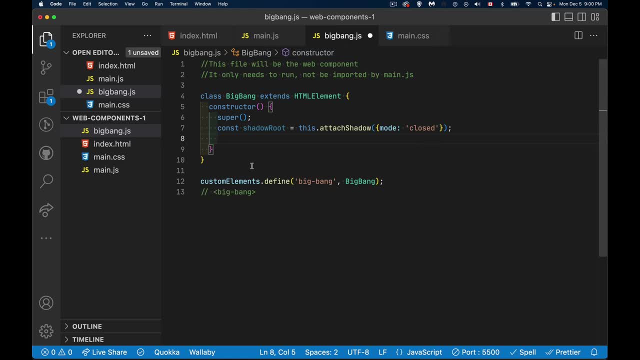 with mode open or closed. so i'm defining a shadow root- that's going to be my container, and then let's put a little bit of html inside of here. so i'll create a div. once we have our element created, we will append this div to our shadow root. 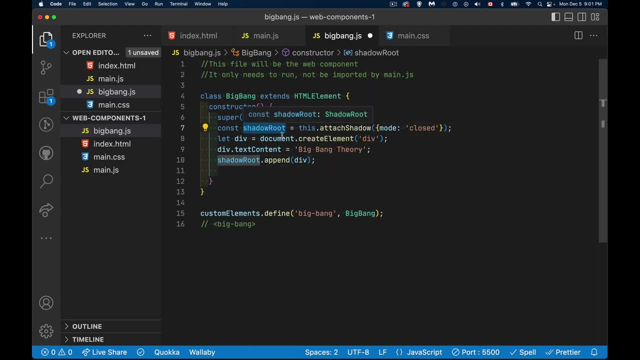 so now we have this shadow root created, we've got a div with some text inside of it. we're going to, We're going to attach the div to this shadow root and there we go, We have created a custom element. That's all it took was for us to define a little bit of HTML. 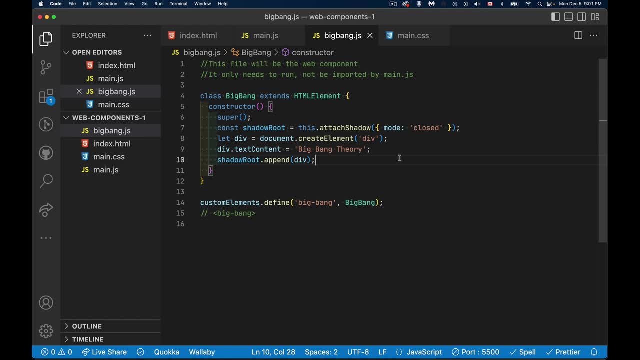 We haven't put any CSS or behaviors in here yet, but we've defined something right here: an HTML element. This is going to be my big bang, which, in the tag, is going to be this: So in here, nothing's happening yet because we haven't added one of these to the screen. 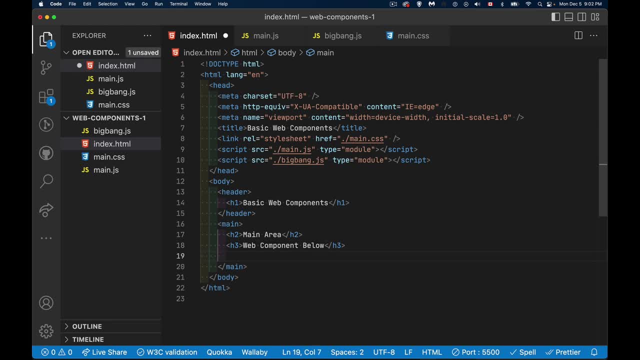 But if I come back to here, I go inside my main element and I'm going to define big bang or I'm going to add big bang to the page. Now, I haven't put any content inside of here, but there it is. 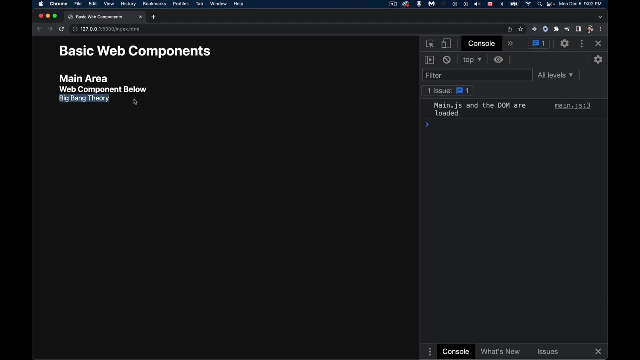 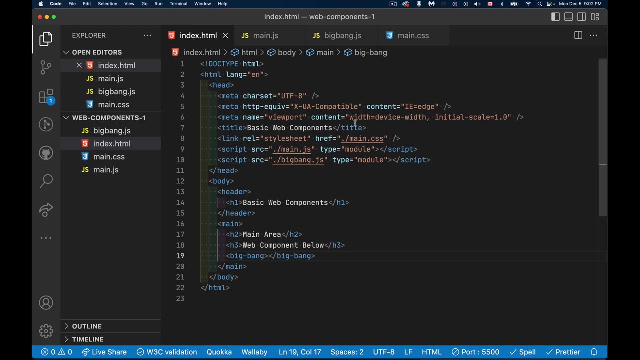 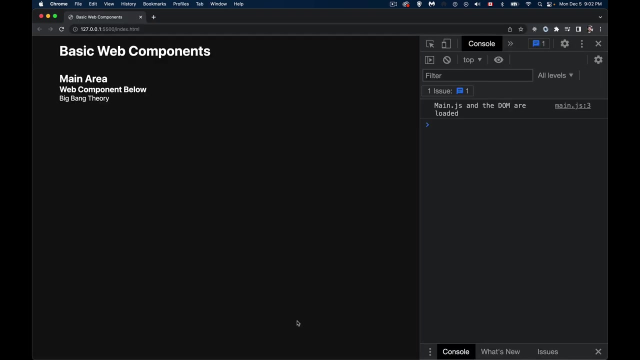 There is my custom component. I have created one and I've added it to the page. by just adding that tag, The text that is in there is built into what we defined inside this script. It doesn't have to be here. In fact, if I do something like this, it's ignored. 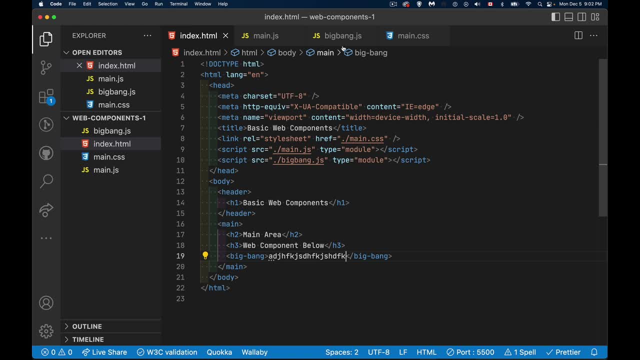 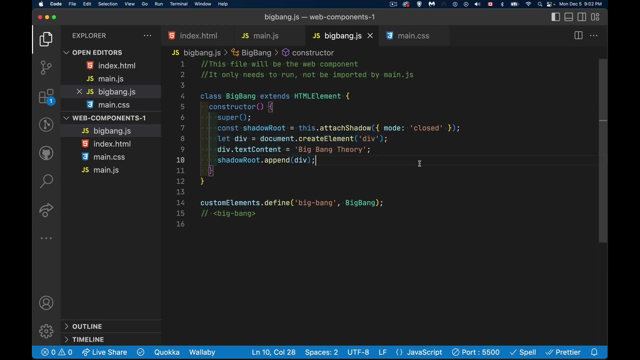 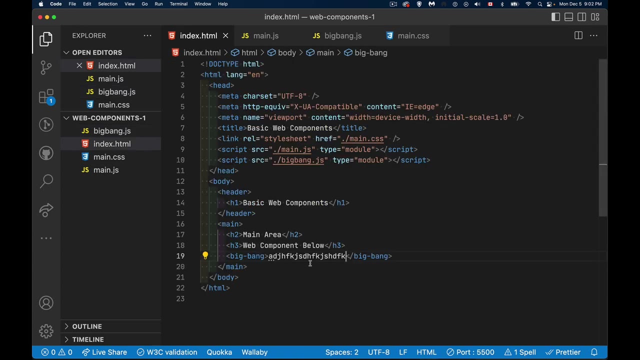 It does not matter what I put inside of here. This defines what this content is, which actually leads us to our next question: How do we get things nested inside? How would I put some content inside of here that becomes part of this custom element? 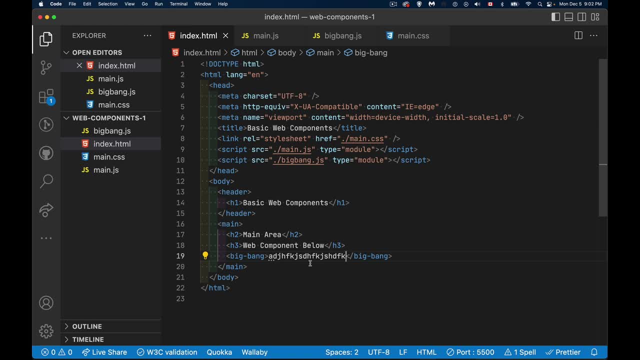 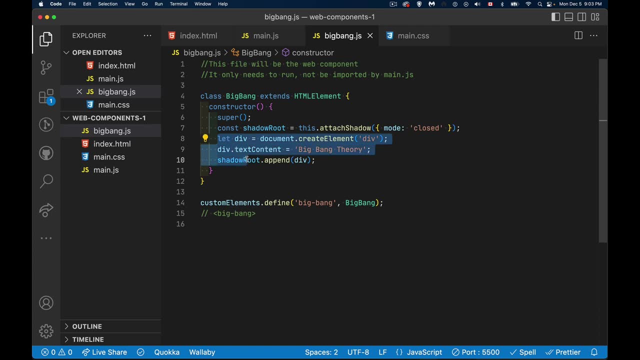 And that's where we have a thing called slots. So we're going to jump into here first and instead of doing this- so I'm going to comment this out- Instead of doing this, where we're defining it all like this, I'm going to actually create. 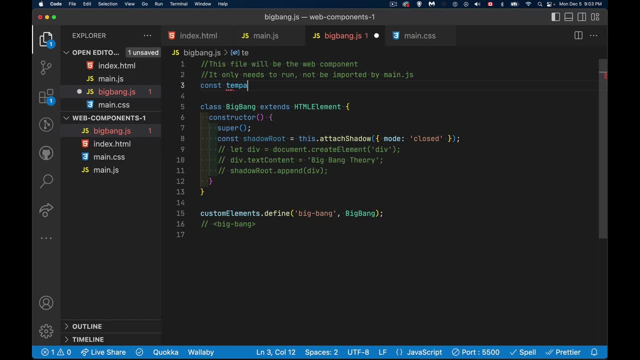 a template, And so we'll call our variable template. So this is an actual HTML element, the template element. I have a video. If you follow the link that's up at the top there, you can see that video as well. So we have a template element, and then I'm going to set its contents right here. 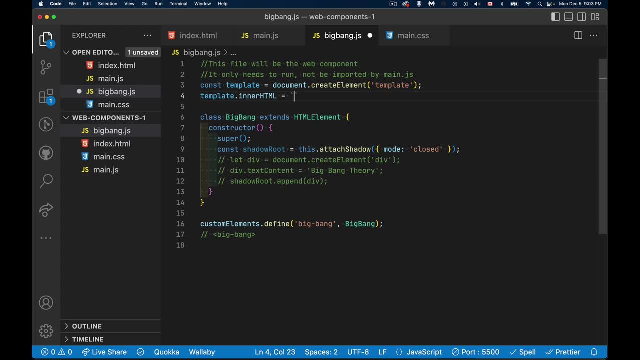 TemplateinnerHTML equals, and I'll use the backtick characters. So, if I want, I could embed variables and other sorts of things. I can have a multi-line string, no problem. And here's the div that we originally had. I'm going to add a little bit more to this one. 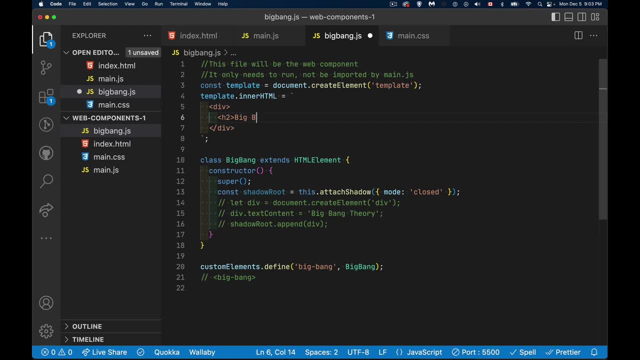 So I'm going to say h2.. Here's my Big Bang Theory header. We could leave it at that. I will come back and add some more here in just a moment, but this is now the template that I'm going to use. 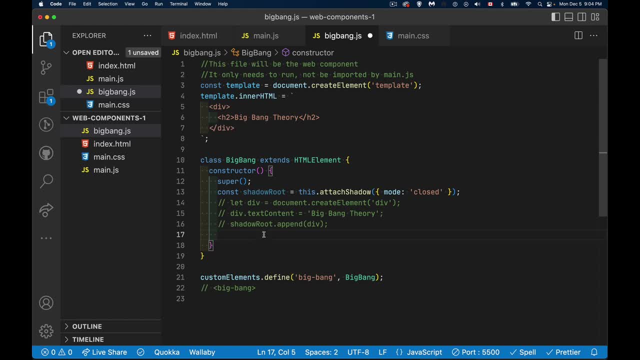 So instead of writing the content here like this, what I'm going to do is I'm going to create a copy of that template, So we'll say templatecontentcloneNode and true Meaning. I don't just want the template element, I want all of its contents, not just the div, but also the h2, everything that's inside. 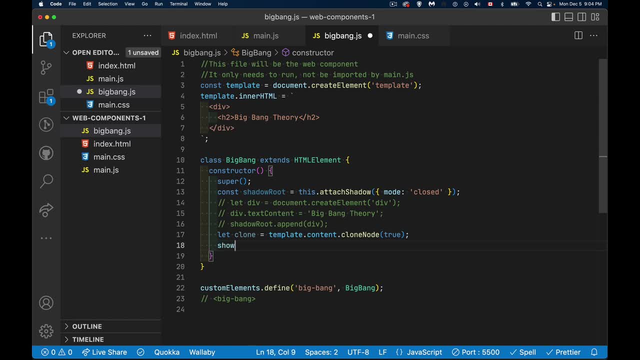 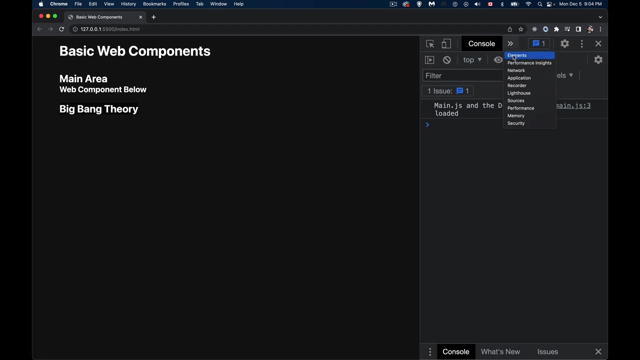 That's what this true means. We're going to go deep inside and we'll do the same thing that we did before: ShadowRootappend our clone, Okay, Okay. So now this is an h2 element, And if we look in elements here in our dev tools, it still says Big Bang. 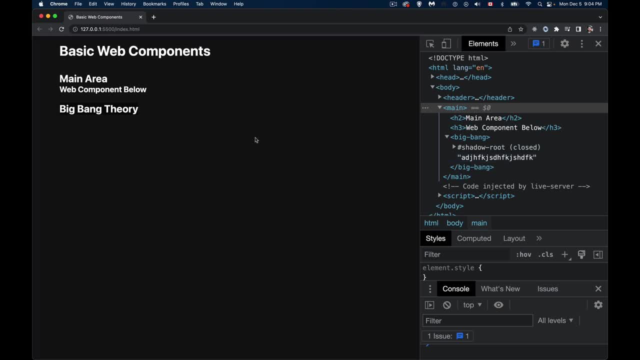 And there's that. There's that text that we actually put into our web page but that's not showing up here. All we're seeing here is this Big Bang. But notice, we do have a closed ShadowRoot. I can open this up and there's the div and there's the h2.. 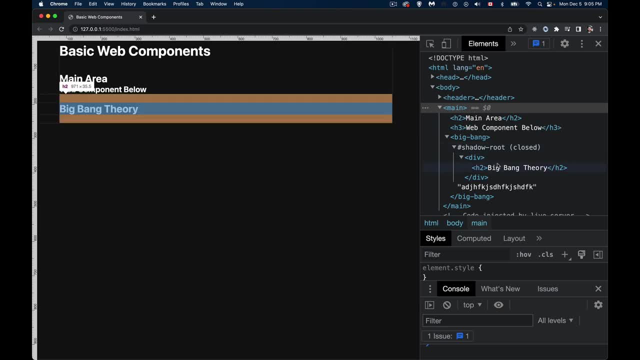 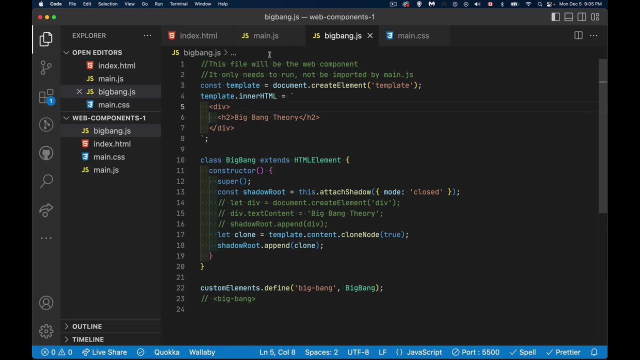 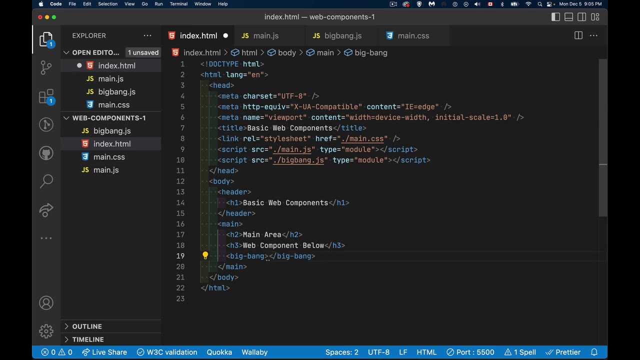 So this is what's inside the ShadowRoot, the stuff that we defined inside of our script. All right, Coming back to this Now, the idea of slots. Well, I want to put some content from here into My Big Bang element. 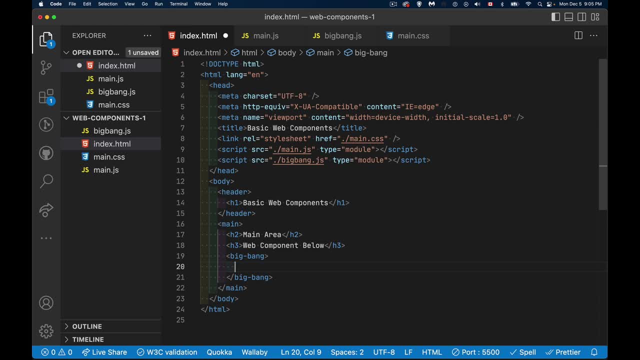 So, just like that, we've got the Big Bang tag itself, but I want to put some text of my own inside of here. So I'm going to create an element. Let's say it's an h2 element and I'll say it's called characters. 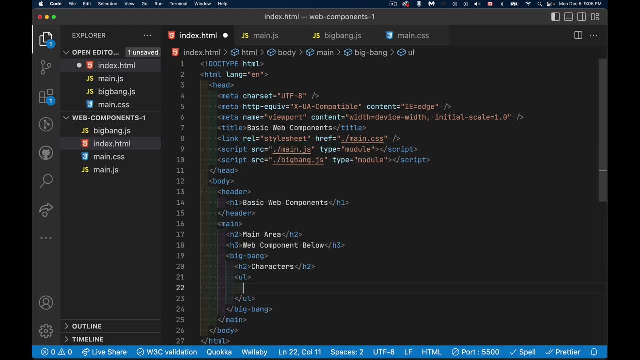 And I'm going to add a list. That should be enough, Just so I have some content here. If I want to be able to use any of this content as part of the finished web component when it's built, what I need to do is I need to come into the element that I want to include and give it a name. 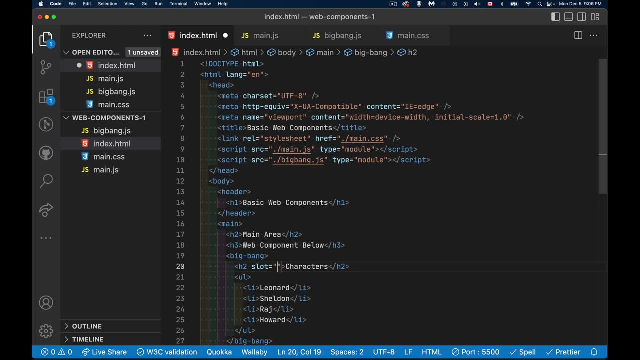 I'm going to say it's going to use the slot which will have the name title, So we'll start with just this h2.. This thing right here is going to be able to be included inside of here. So when we come over here, 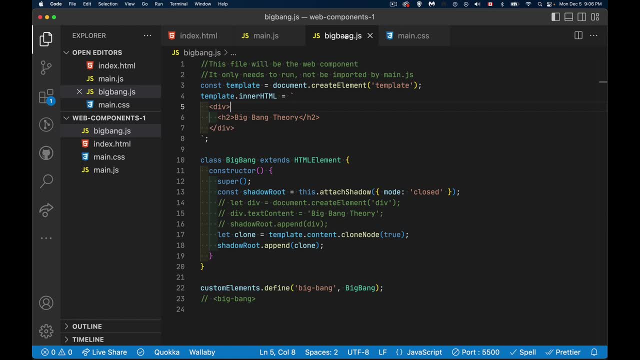 So when we come over into our template that we were defining up at the top more than just this h2 and actually let's make this an h1 because we're going to be adding an h2.. I'm going to say that I'm going to define a slot with the name title, like this: 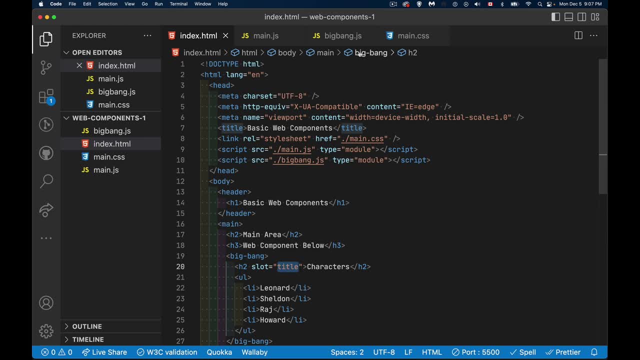 So this slot title right here is going to match up with slot title. So this slot title right here is going to match up with slot title. So this slot title right here is going to match up with slot title. So this slot title right here is going to match up with slot name title. 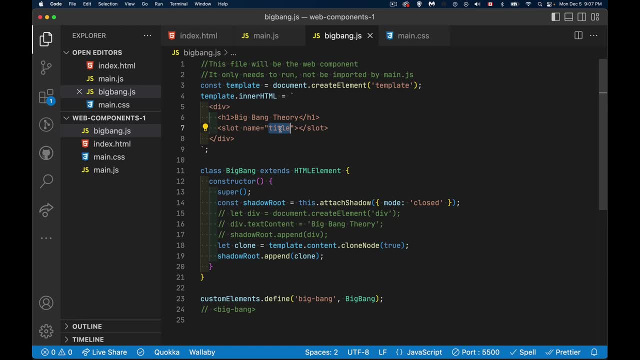 So this slot title right here is going to match up with slot name title. So this slot title right here is going to match up with slot name title. So the title in the two places, that's what connects this together. So the title in the two places, that's what connects this together. 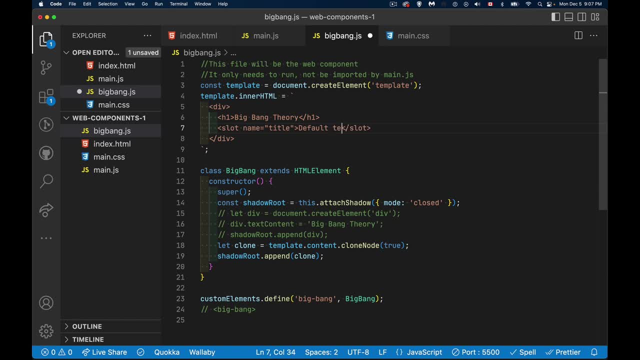 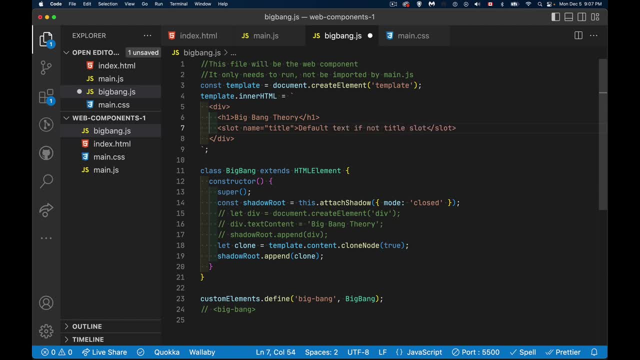 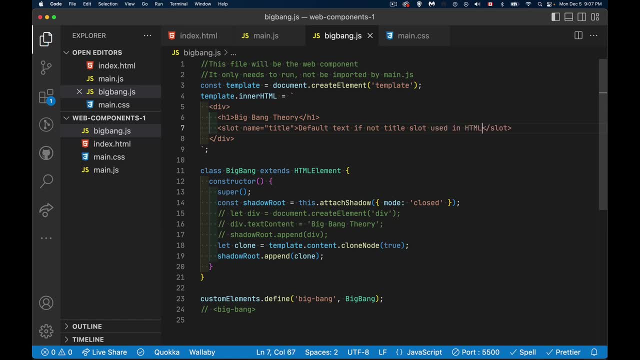 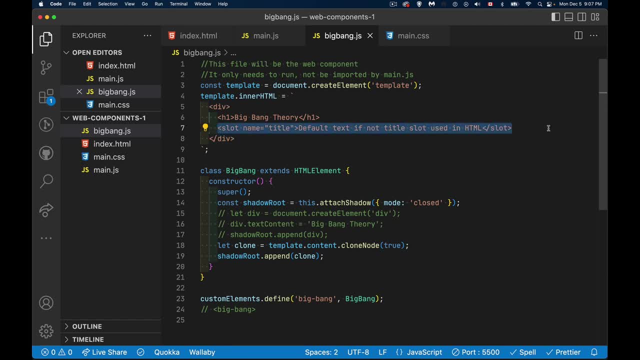 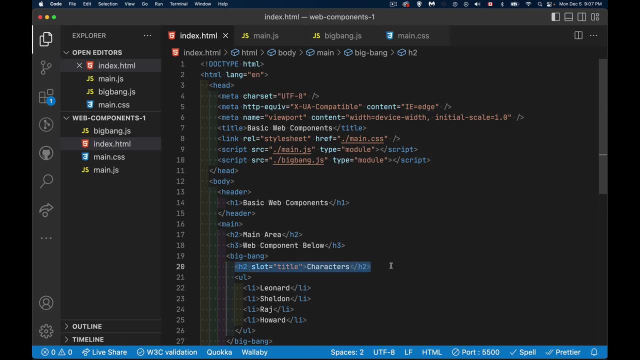 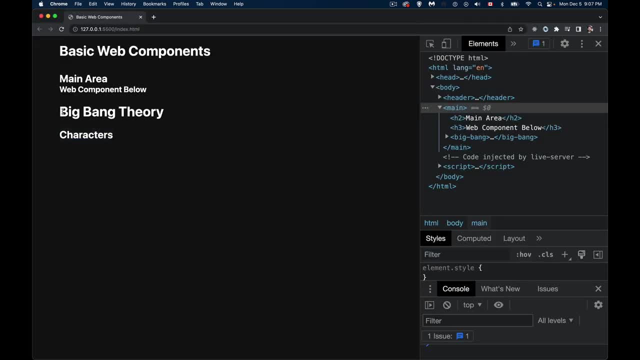 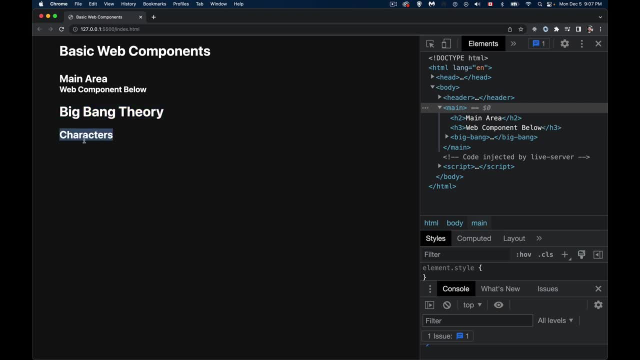 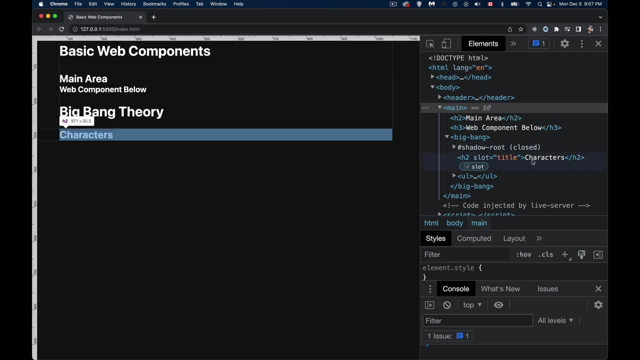 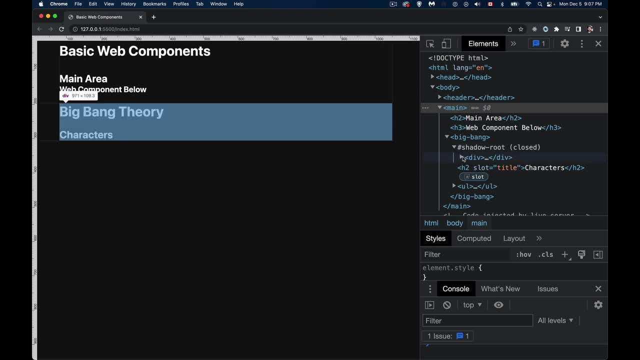 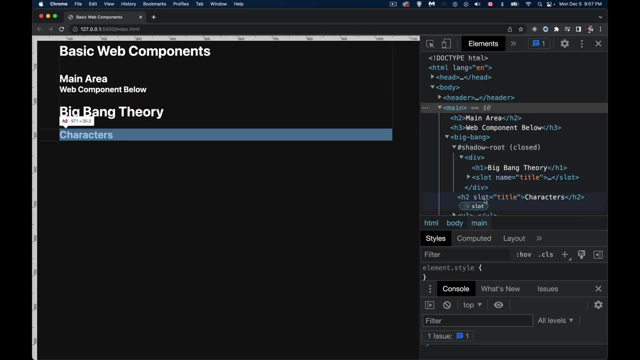 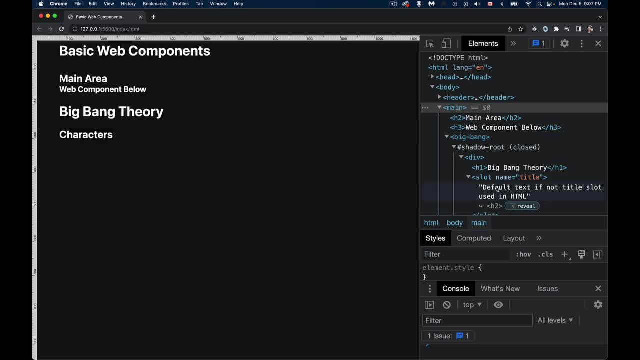 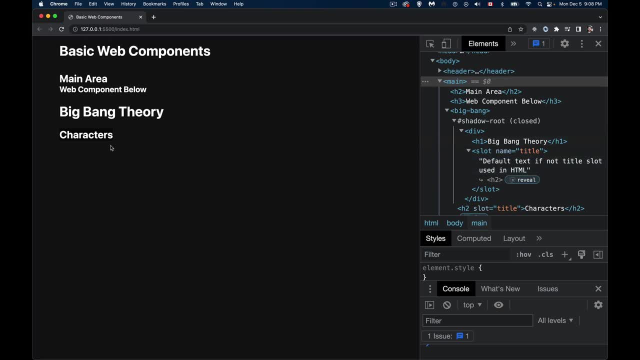 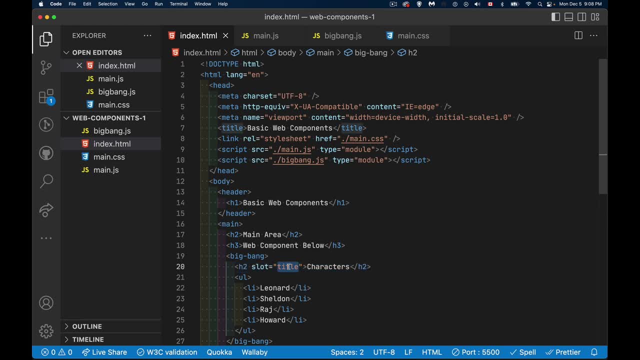 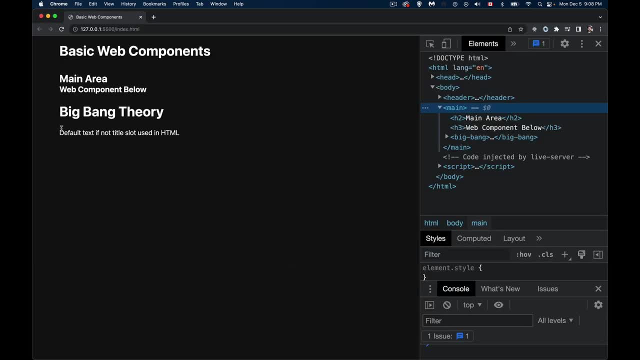 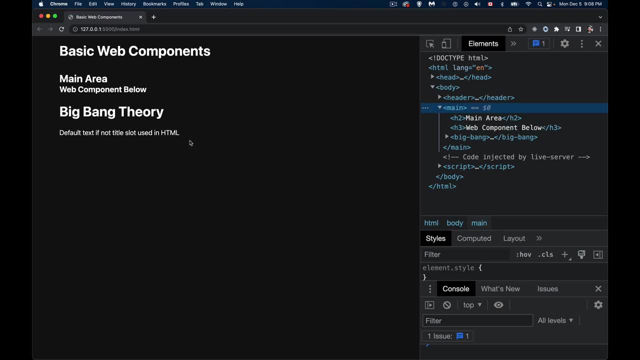 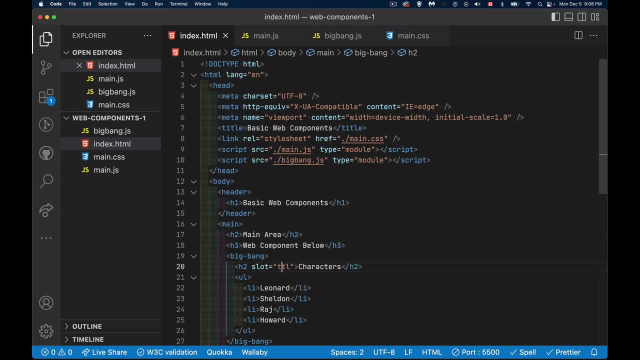 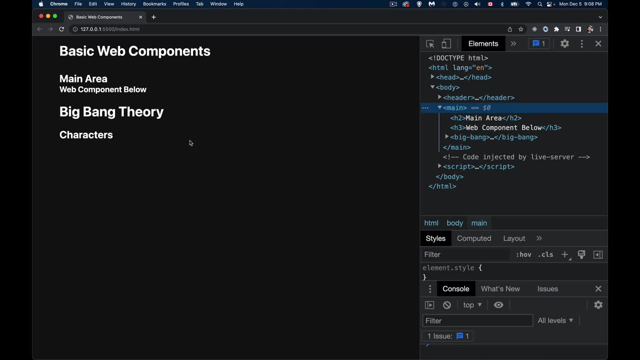 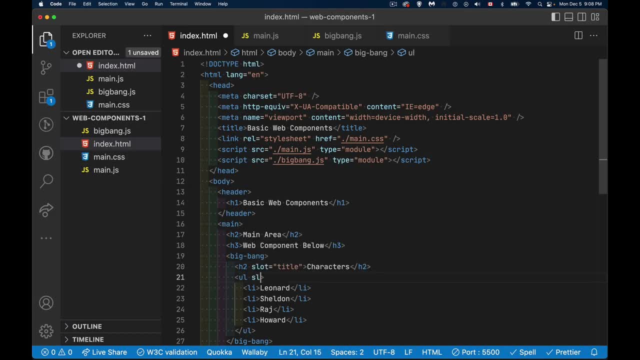 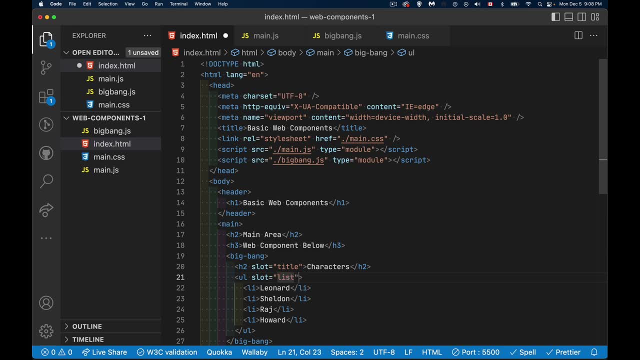 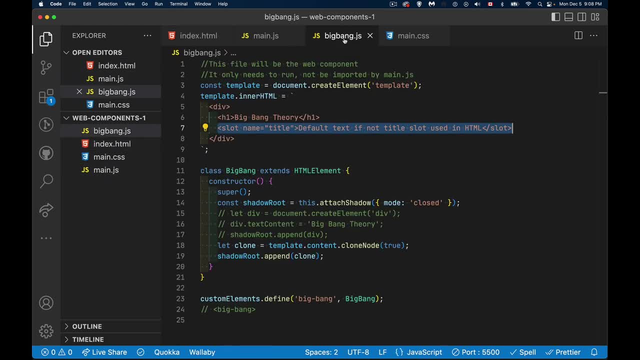 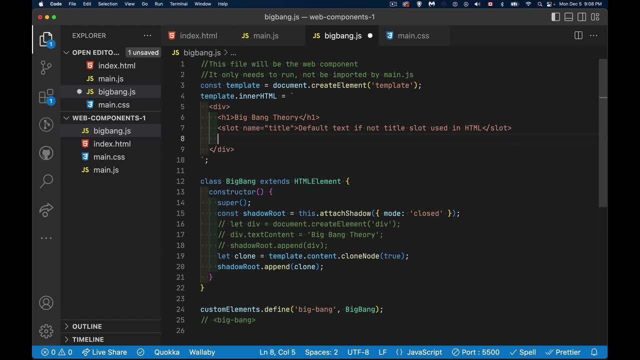 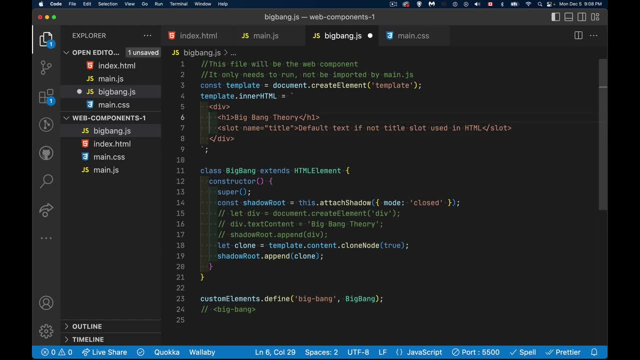 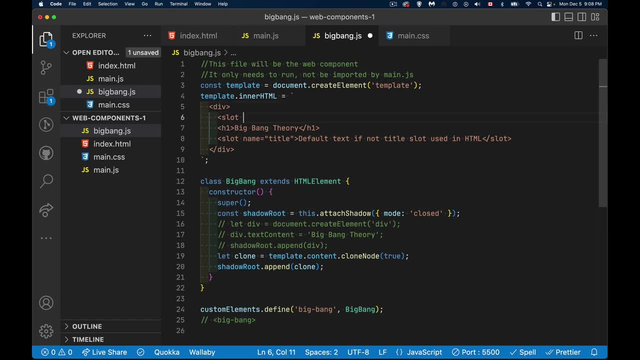 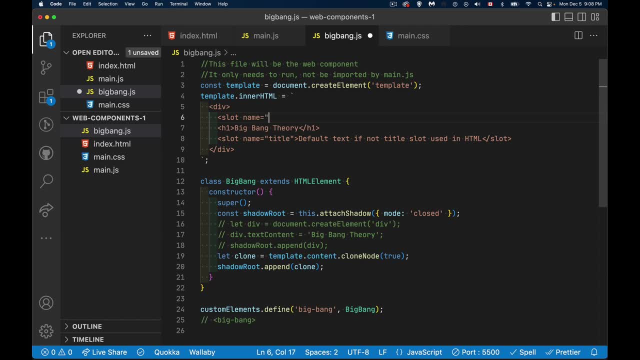 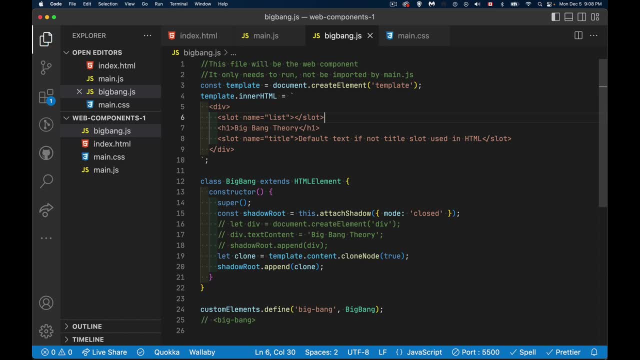 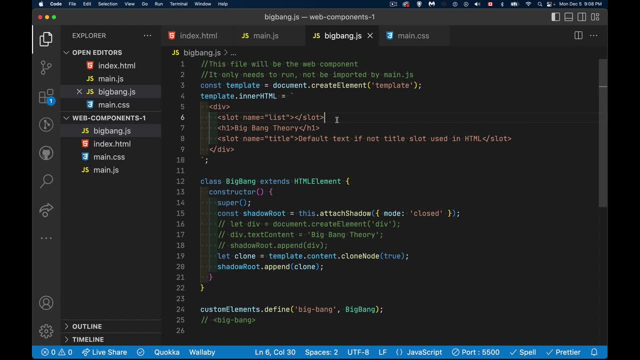 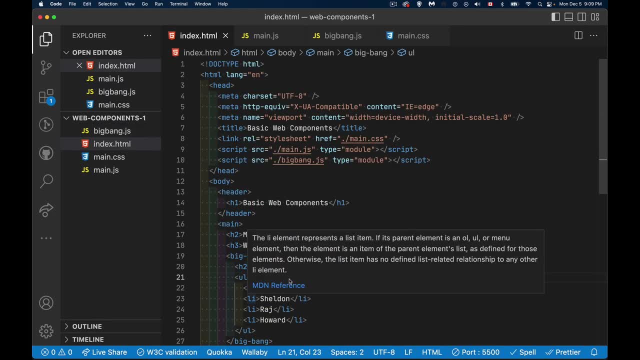 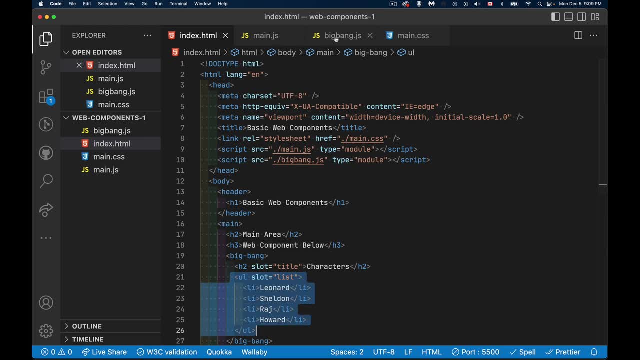 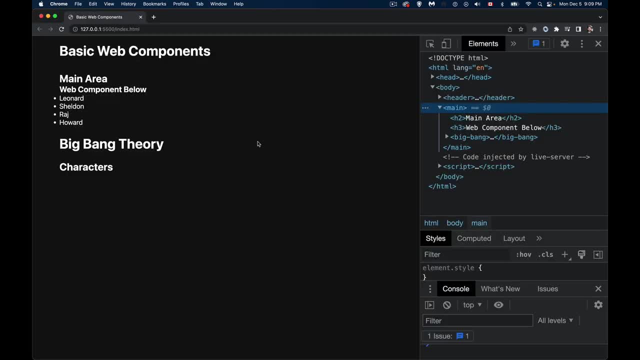 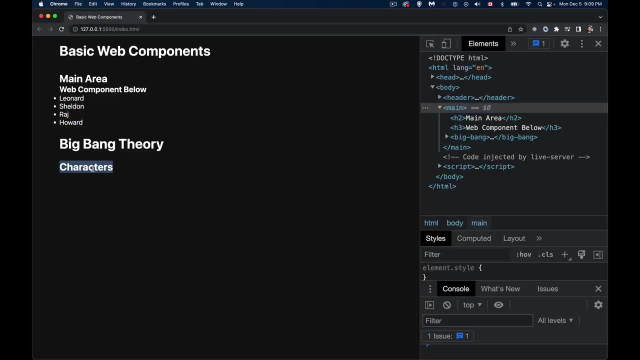 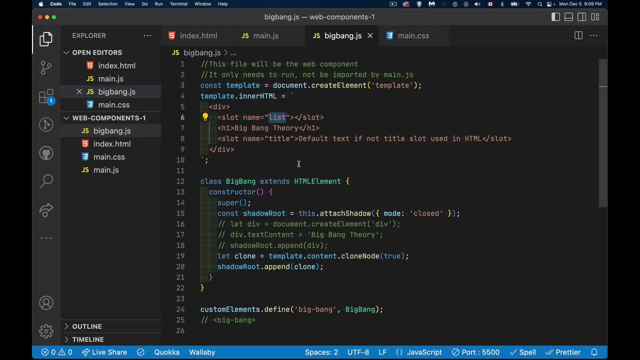 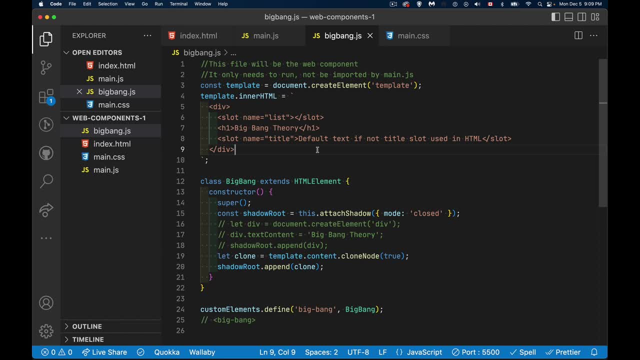 And we could have some default text if no title slot used in HTML. And we couldn't have some default text if no title slot used in HTML. And we could have some default text if no title slot used in HTML. And we could have some default text if no title slot used in HTML. 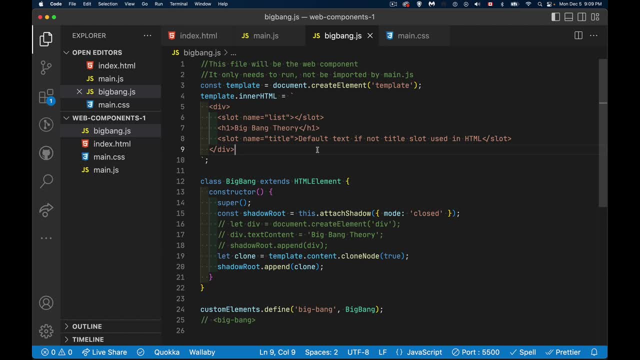 And I just wanted to show this little summary- and I didn't mean to ramble on inside of here, And that's it. That is the fundamentals of how you can create web components. Now there is more to this. Now, there is more to this.